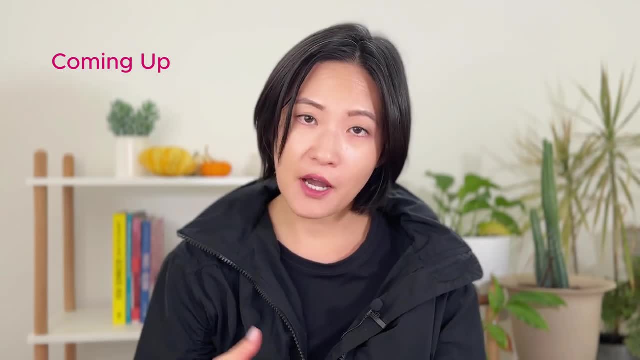 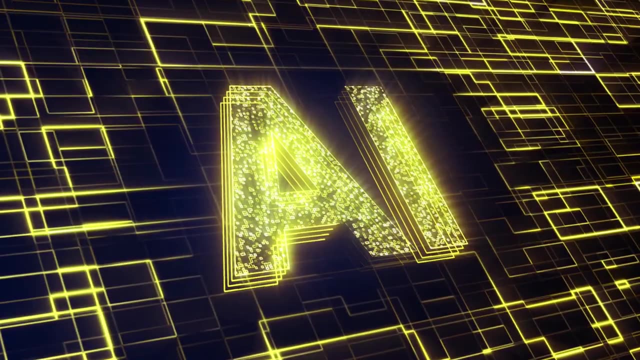 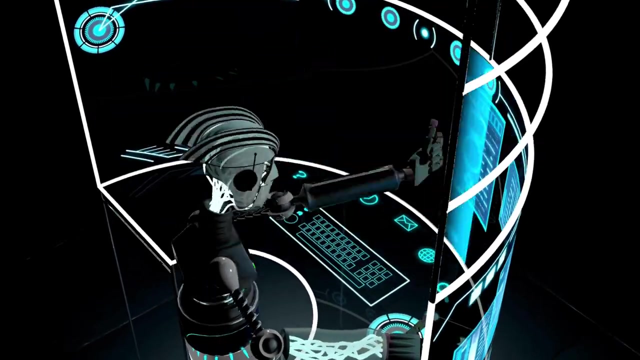 Instead of falling into the rabbit hole of tutorial hell, learning by doing is the way to go. This technique is something that everyone can use. Let's jump right into the study plan. With the advancements in AI and machine learning making headlines daily, it's evident that these technologies are shaping our future. AI is on track to generate 13 trillion. 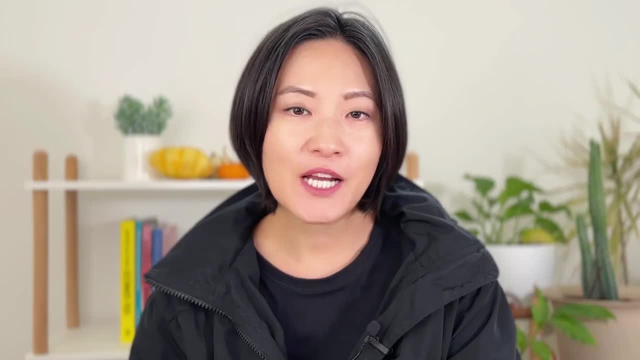 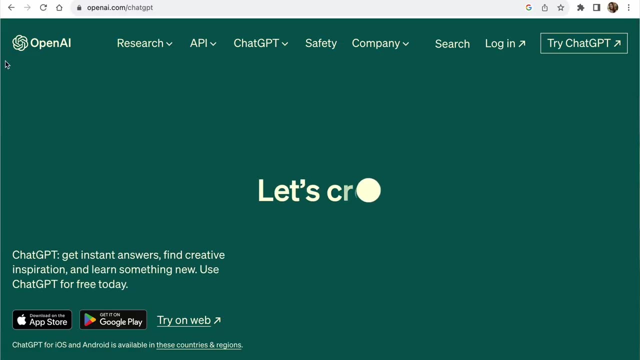 dollars in economic value by year 2030.. Let's talk about how you can tap into this market and ride the wave of AI and machine learning using ChatGPT. You see, these days I use ChatGPT for just about everything. It's my go-to source for knowledge, assistance and inspiration. It's 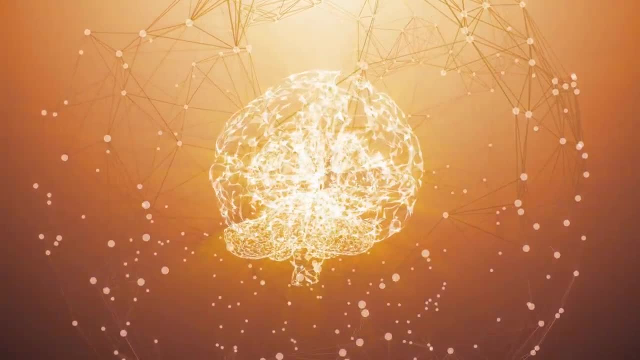 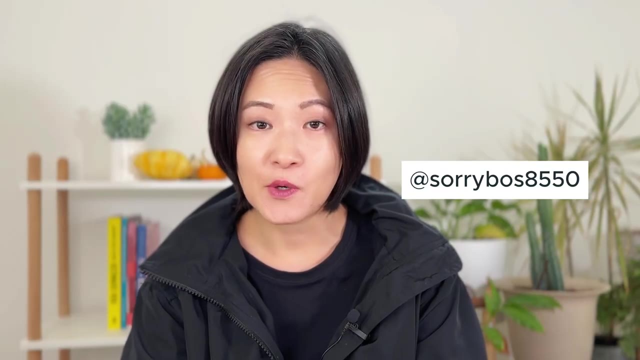 kind of like having that brilliant friend who not only has all the answers but can also explain the most difficult concepts in the world. Recently, one of our viewers, sorryboss8550, asked a really great question in the comments. It was about learning AI through more hands-on projects. 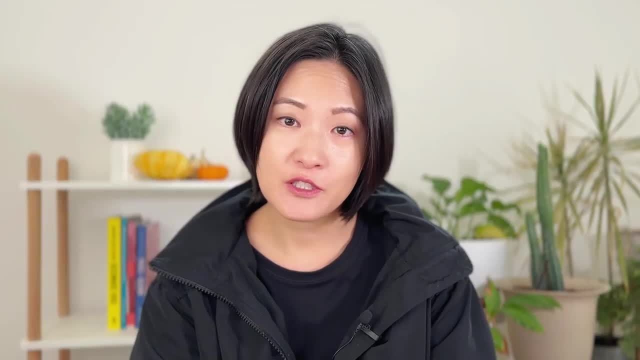 instead of falling into the rabbit hole of tutorial hell. Thanks so much for asking the question And if you have any questions, feel free to ask them in the comments below. And if you have any questions, feel free to ask them in the comments below. And if you have any. 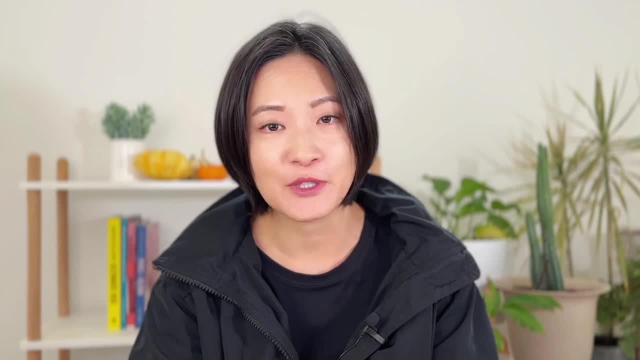 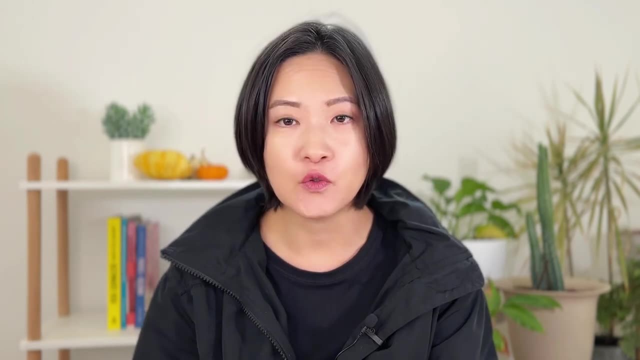 questions, drop them in the comments and I'll make videos around them in the future. I have the perfect solution for hands-on learning that I'm excited to share today. This technique is something that everyone can use on pretty much any topic, whether it's AI. 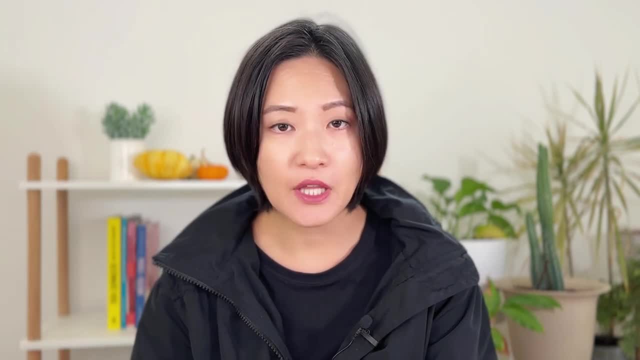 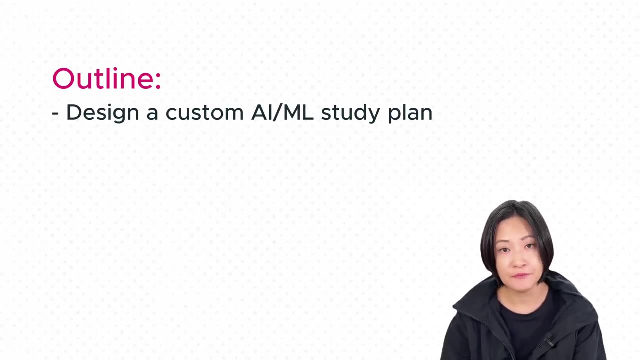 or machine learning or even something completely different. You can pretty much build any tailor-made study plan using this method. In this video, we're going to design a custom AI machine learning study plan together. We'll also talk about how you can build a. 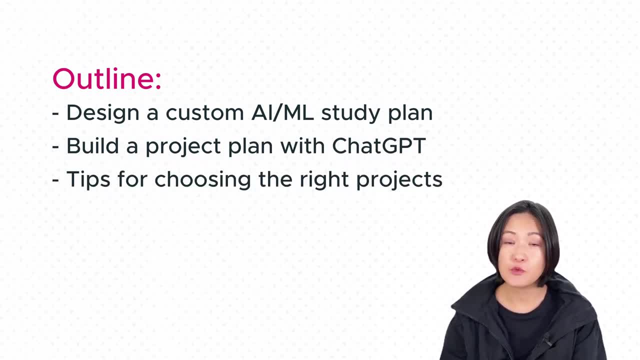 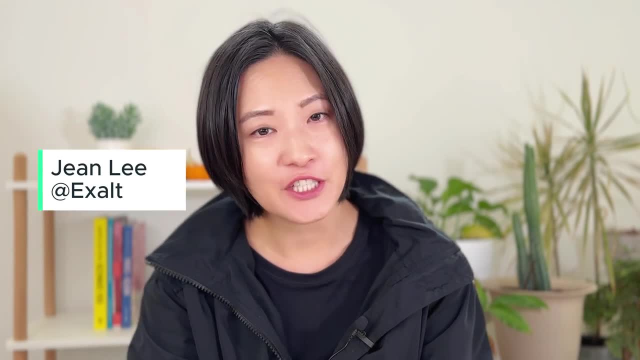 project plan using ChatGPT. I'll share some tips for choosing the right project for yourself, and I'll throw in a quick bonus on how you can showcase your projects on GitHub. By the way, if you're new here, I'm Jane, your trusted engineering mentor. I was an early 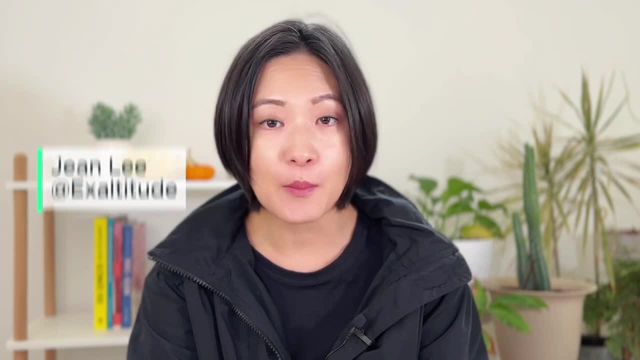 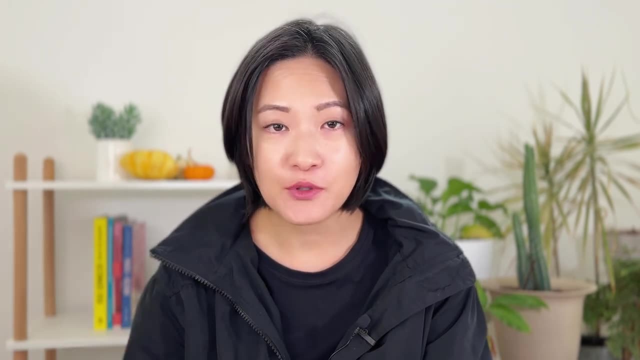 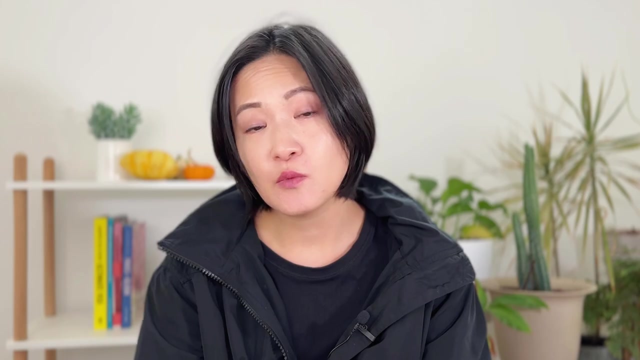 engineer at WhatsApp and an engineering manager at Facebook, now Meta, with over 15 years of experience working in tech. Back when I was studying for computer science, resources like we have today were pretty scarce. I suffered through the boring textbooks and terrible tutorials, which was not the most effective way to learn. ChatGPT is by now a familiar name for 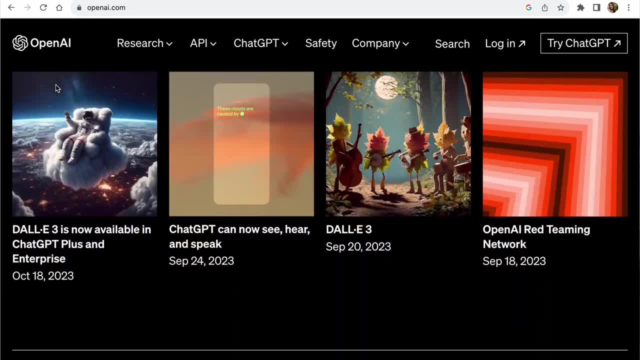 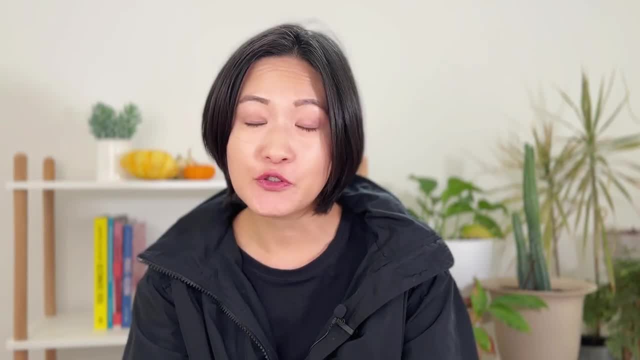 most of you. This advanced AI language model developed by OpenAI is exceptional at comprehending and generating human-like text. Don't worry, I won't bore you with an introductory lecture about ChatGPT. I'm sure most of you are familiar with it already and there's already tons of. 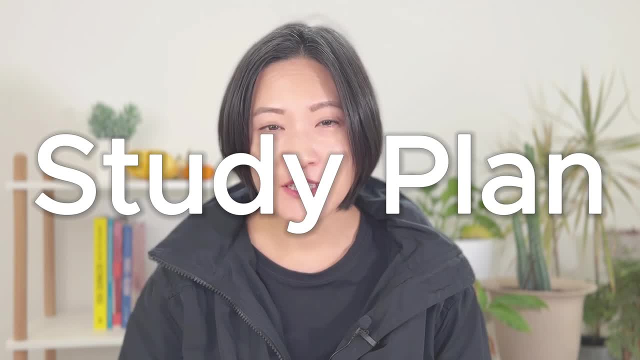 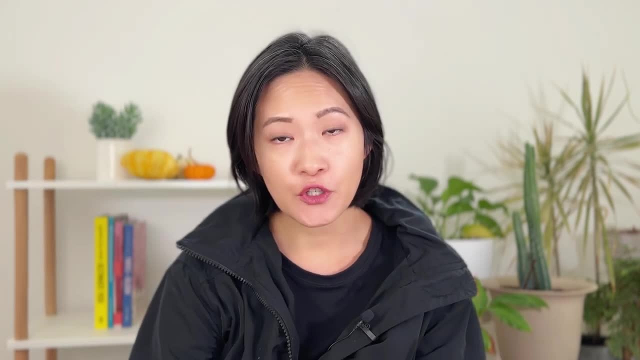 information available for you online. With that, let's jump right into the study plan Now. when you first engage with ChatGPT, your instinct might be to start with a simple request. For example, you can ask: give me a study plan for learning AI and machine learning. 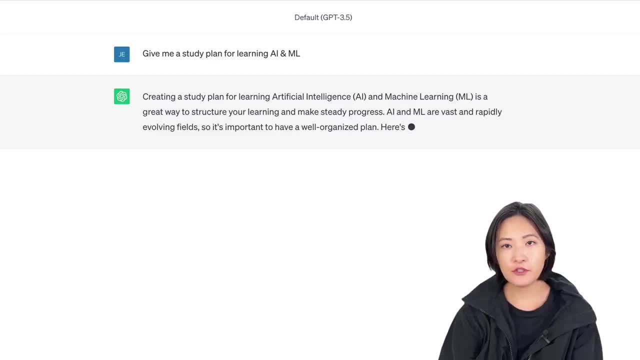 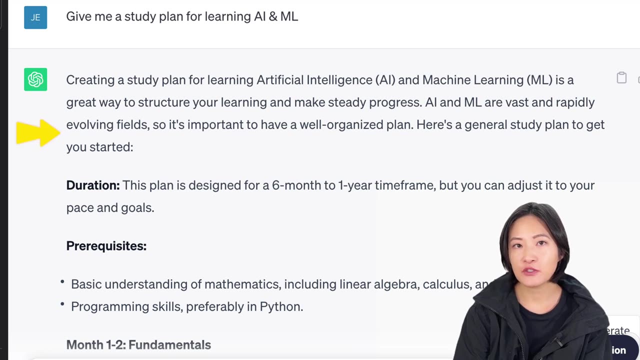 ChatGPT may give you an answer like this. Creating a study plan for learning, artificial intelligence and machine learning is a great way to structure your learning. AI and machine learning are fast and rapidly evolving fields, so it's important to have a well-organized plan. Here's: 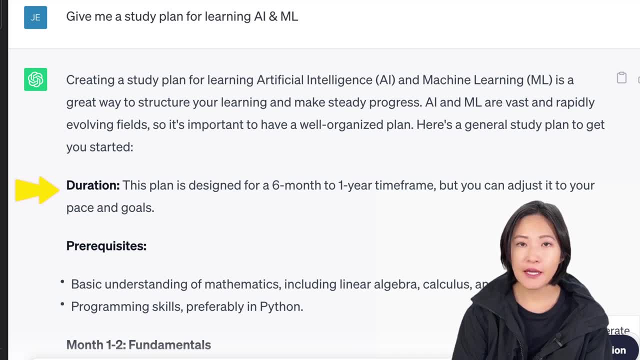 a general study plan for you and I will suggest a duration. This plan is designed for six months to one year time frame, but you can adjust it to your pace and goals. Pre-reqs are basic understanding of math, including linear algebra, calculus and probability. Those are great. 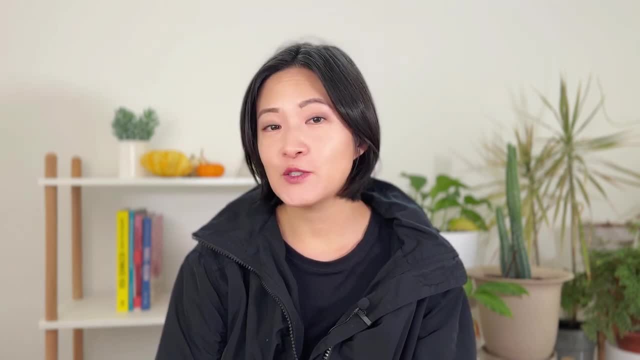 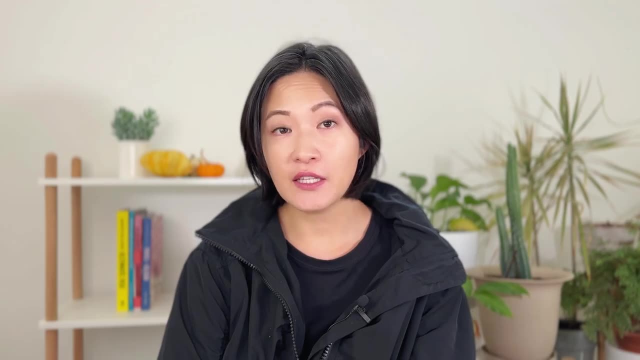 for beginners, but if you're new to programming, it recommends Python, which is great because Python is my choice of language. The study plan is not bad, but it's pretty basic and pretty broad. Let's work on something better. As with any software, quality of your input will directly 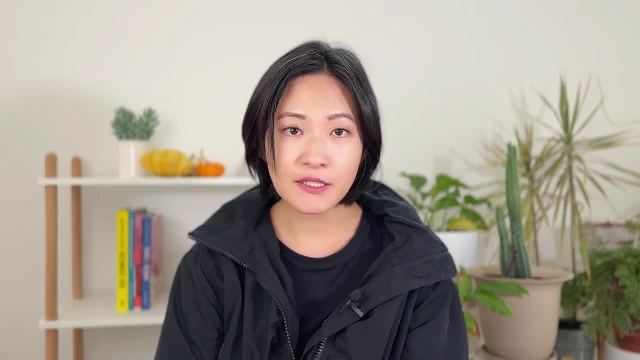 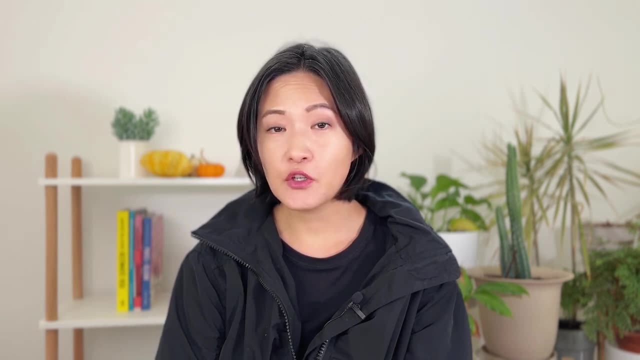 impact the quality of the output. Remember, the more specific and detailed your request, the better the result will be. It's like fine-tuning your search query but honestly, if you really want to learn machine learning as a beginner, it would probably take more than a year. 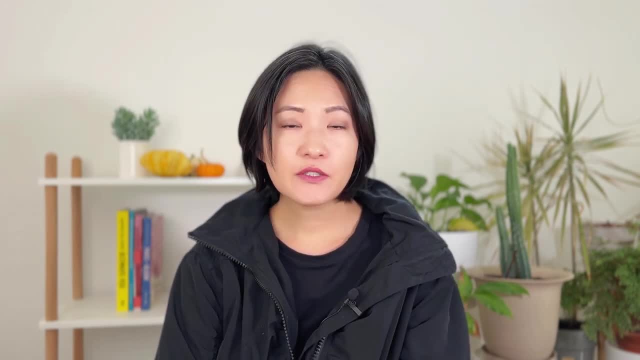 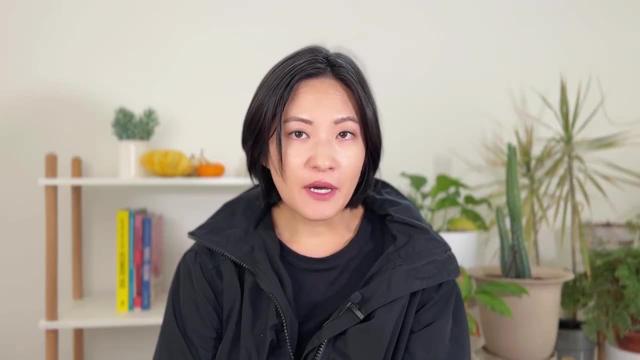 to learn it, But for this study plan, let's see what the study plan is like. For example, if you're looking for a six-month plan, let's refine our request. Give me a six-month study plan for learning AI and machine learning. This response is a little better, but it's still way too broad. 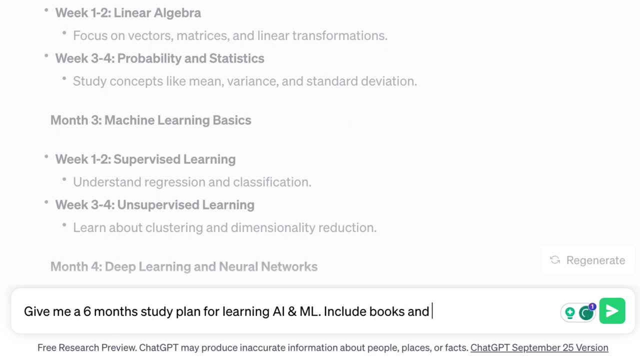 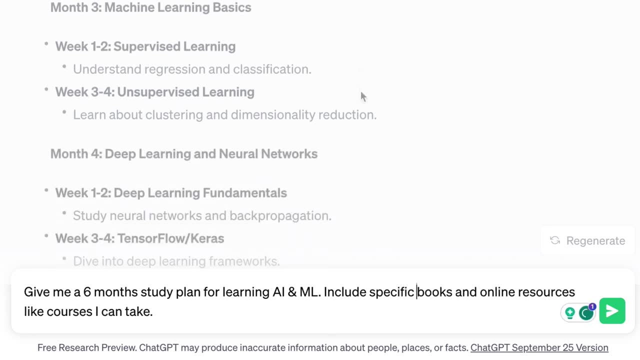 Let's make it even more detailed. Give me a six-month study plan for learning AI and machine learning. Include specific books and online resources. like courses I can take, I would like free courses if possible, And here's what ChatGPT came up with. 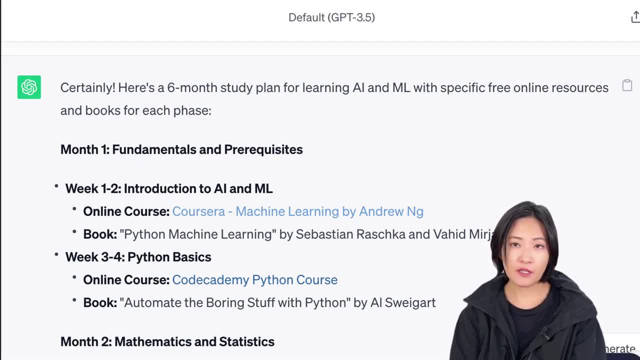 In week one to two: introduction to AI and machine learning: online courses by Coursera. machine learning by Andrew Ng. book recommendation is Python machine learning. Week three to four is Python basics online course by Code Academy. Book recommendation is automate the. 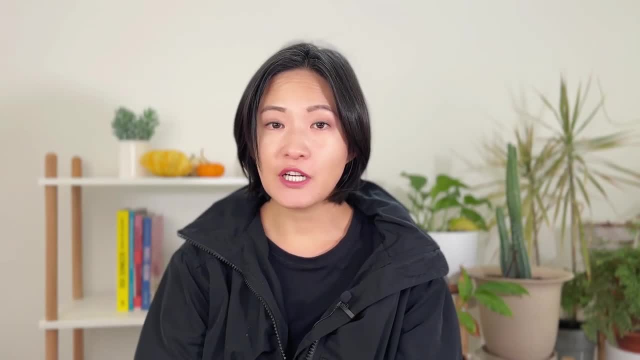 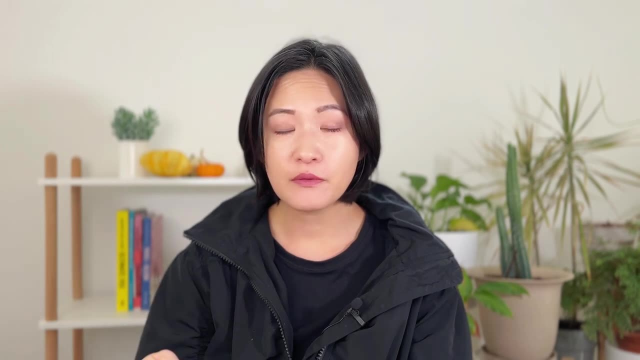 boring stuff with Python. Now this study plan is pretty aggressive. Remember the original plan was for six to 12 months. right, If you're new to Python or machine learning, you would probably want to double the lengths of each topic, For example, instead of one to two weeks. 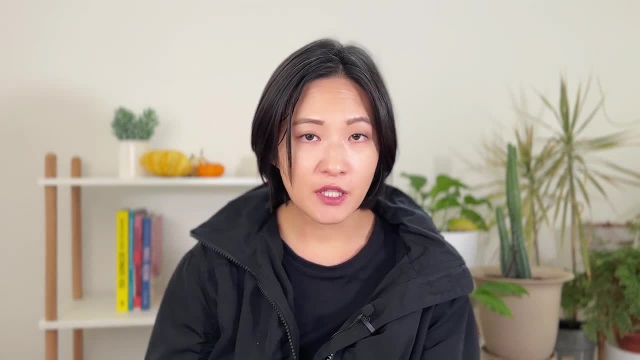 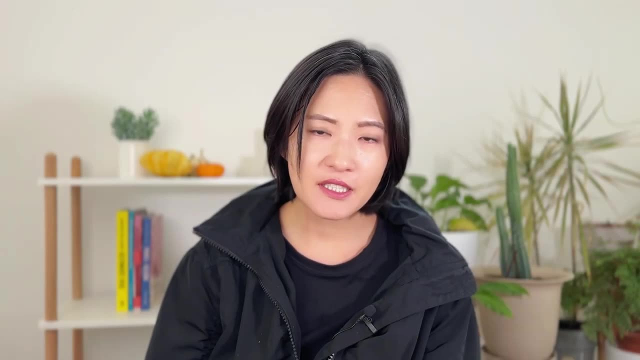 make it a one-month goal. I like the book and the free resource recommendations. However, I do see that Coursera's machine learning by Andrew Ng was recommended twice, which is not too bad, because it is a great course, so it wouldn't hurt to study it for. 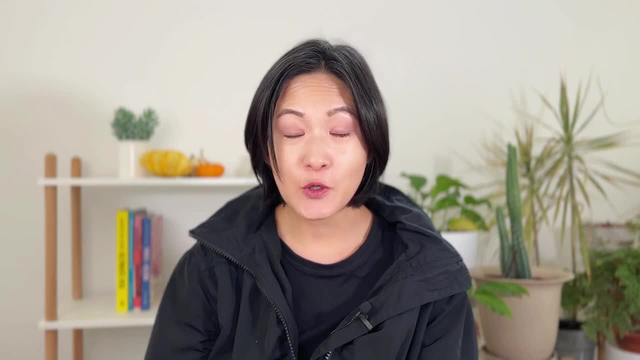 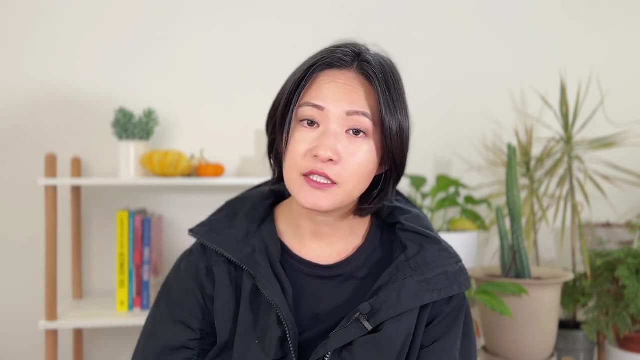 a longer period of time. Some of these books are textbooks that would take you an entire semester to study. So it's up to you if you want to actually read through the entire book, or you can reference them as needed. Month six is recommended for capstone projects, and 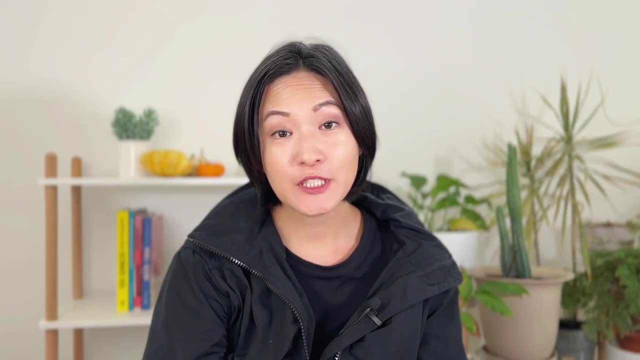 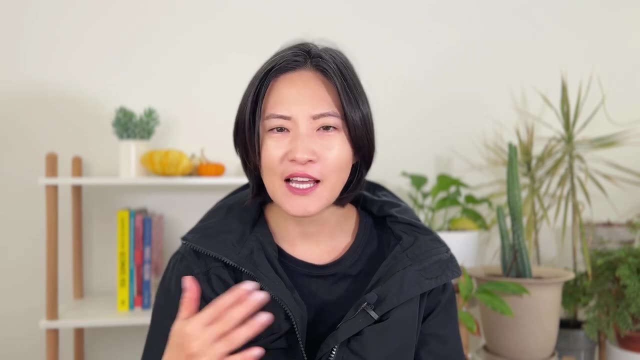 applications. It's a great start, but it's too vague. Back when I was in college, I struggled with the theory-heavy classes and I was wondering why I was learning this and how they would help me in the future. So for me, learning by doing is the way to go, If you're like me. this next section is: 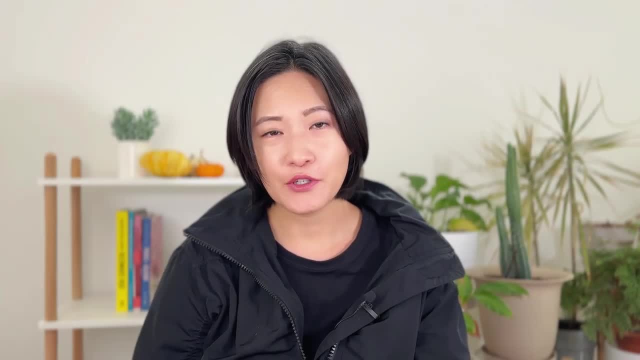 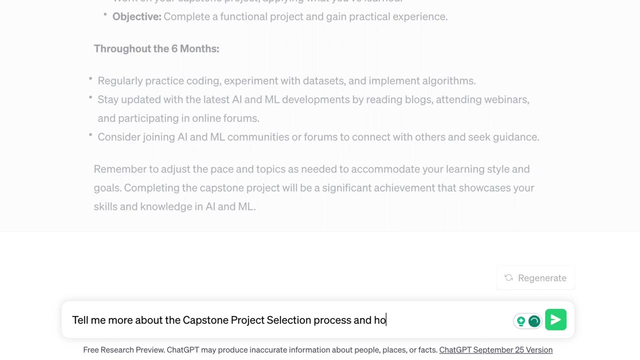 for you. We'll focus on learning by doing and how it can make learning a lot more engaging and practical. So I'm going to ask this new prompt: tell me more about the capstone project selection process and how I can approach it. It says step one is to define your interests. Start by. 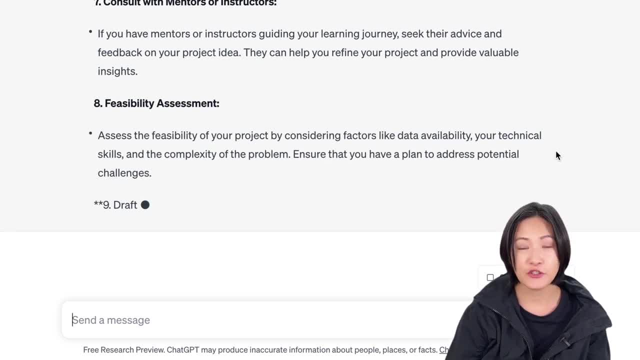 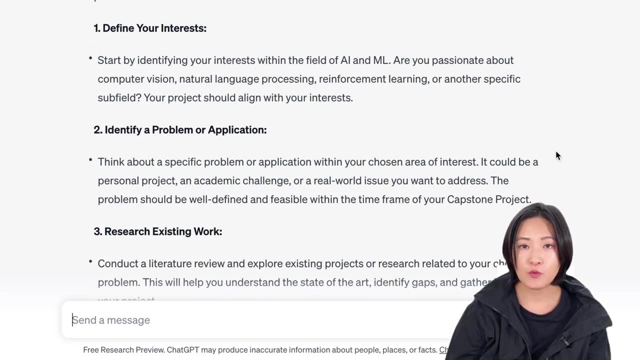 identifying your interests within the field of AI and machine learning. Are you passionate about computer vision, natural language processing or any other specific subfield? Your project should align with your interests. Step two is to identify a problem or application. Think about a specific. 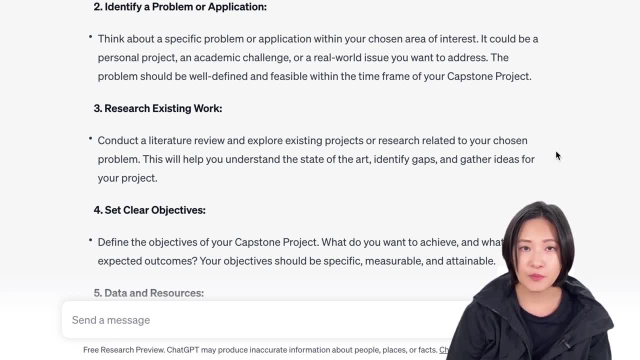 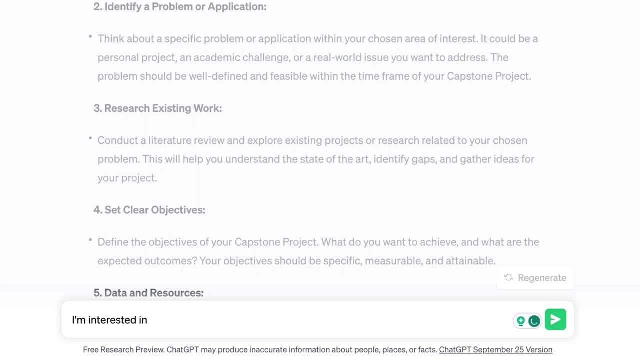 problem or application within your chosen area of interest. It could be a personal project, et cetera. This stage is all about choosing something that excites you. So, as the next prompt, I'm going to ask: I'm interested in exploring natural language processing. 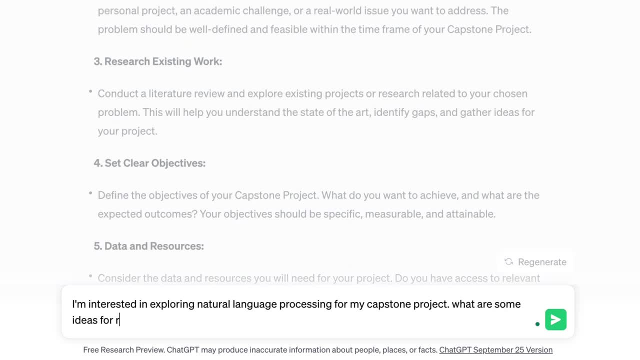 That's the interest that I chose for this example For my capstone project. what are some ideas for problems or applications? Give me ideas for personal projects I can work on. This is for those of you who have absolutely no idea where to start Now. I really love this result because 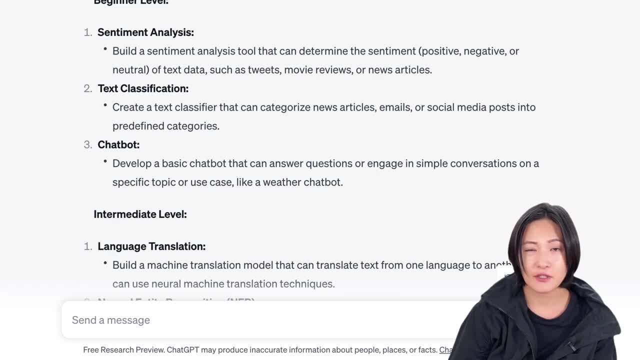 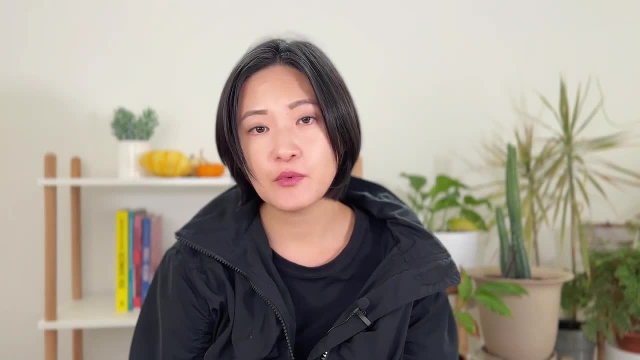 it even includes beginner, intermediate, advanced and research level projects. So let's look at the suggestions. Now let's pick an interesting project. I get a lot of questions from people who are not sure which projects to choose. Here's some of my tips on how to choose. 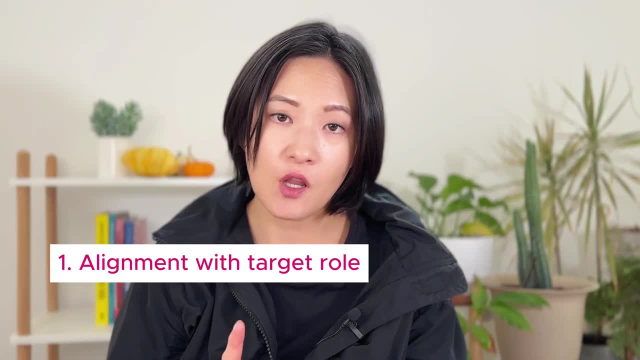 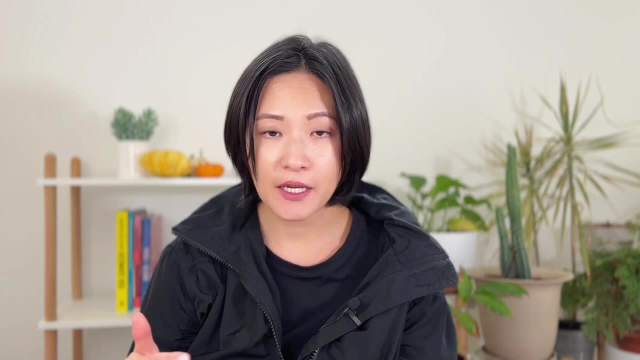 the right projects. Tip number one is to make sure the projects align with your target roles. What type of engineering do you want to go into? Let's say you want to dive into roles like front end or backend, or mobile app. Each of these roles come with specific tech stacks. So if you want to 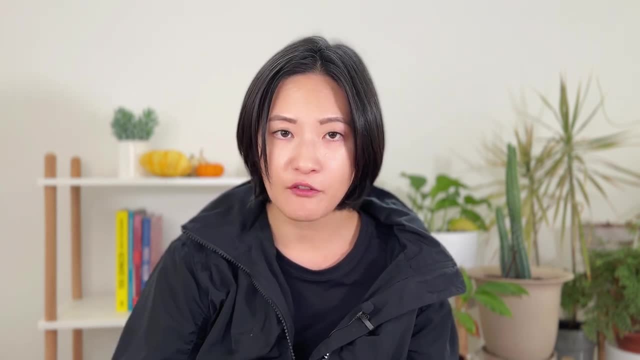 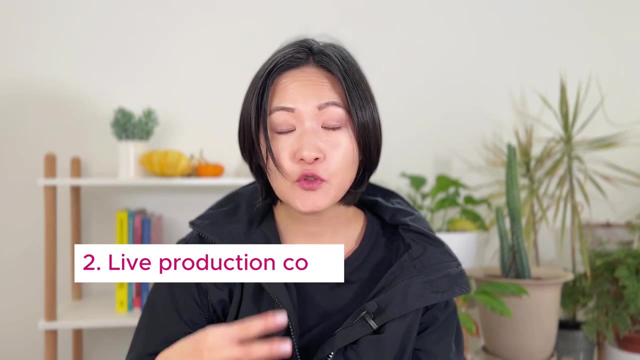 be a front end developer, choose projects that are going to show off your front end skills. If you want to be a mobile developer, go build a mobile application. Pretty straightforward. Number two is to work on real life production code. So if it's a mobile app, put it on the. 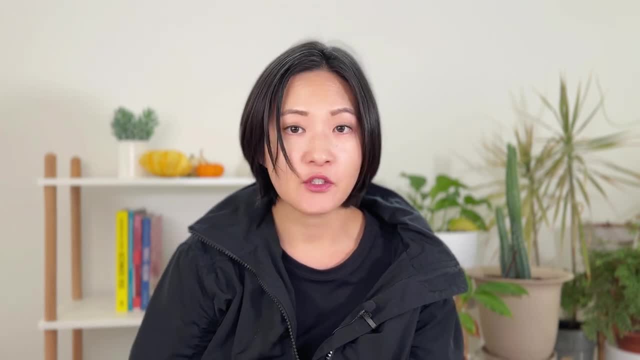 app store. It should be live and accessible so anyone can download it and use it. If your experience is limited, you can use the app store. If it's a mobile app, you can use the app store. If it's limited to school environment or classroom setting, that's not very impressive. 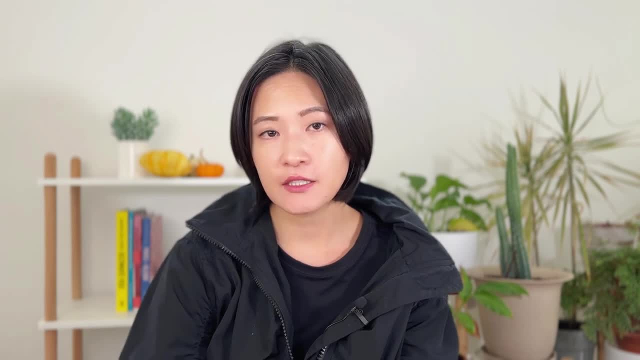 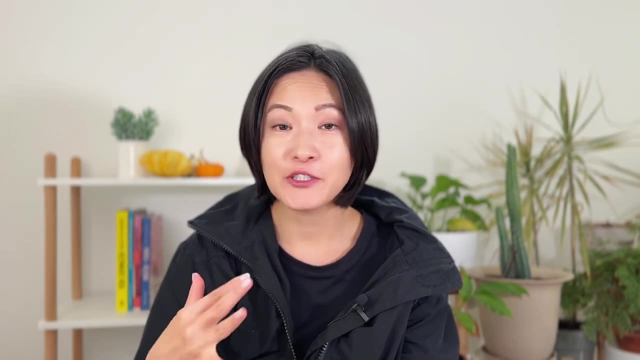 You want to show that your project is more than just an exercise. It should be a practical application. Tip number three is to solve real life problems. Your projects don't have to be groundbreaking or entirely new. You can even take existing ideas and add your twist to it, or 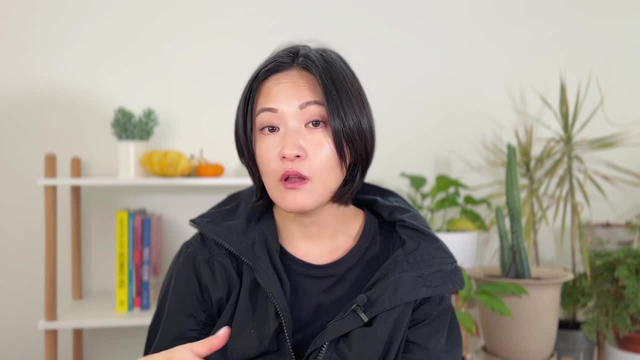 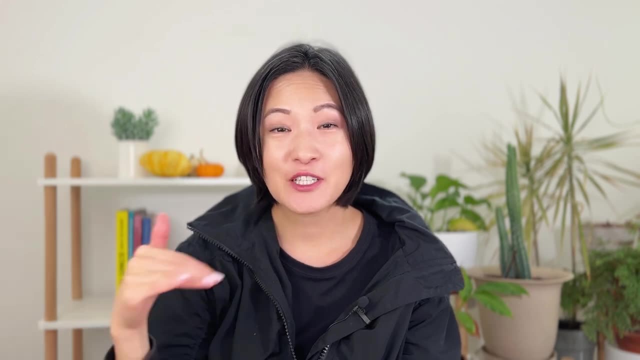 build a smaller selection of features. It will make your work a lot more meaningful when other people are using it and you're actually solving real life problems. What are some projects that you're working on? Share them in the comments. I would love to hear about them. Now let's get back to ChatGPT to build an actual project plan. 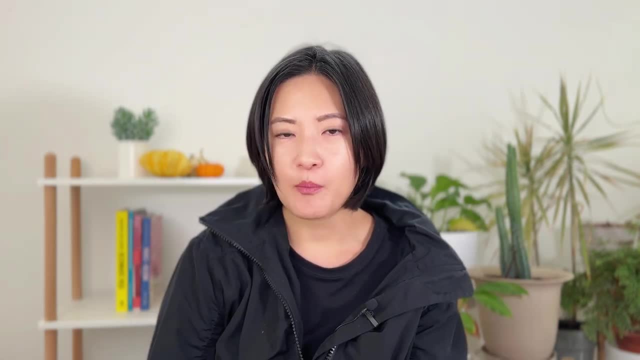 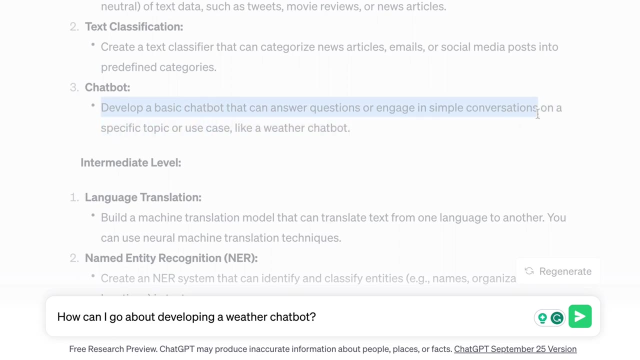 From the beginning level project ideas. I like the weather chatbot idea. So first I can ask: how can I develop a basic chatbot that can answer questions or engage in simple conversations like what's today's weather? Then ChatGPT gave me a 14 step process, which is pretty practical. 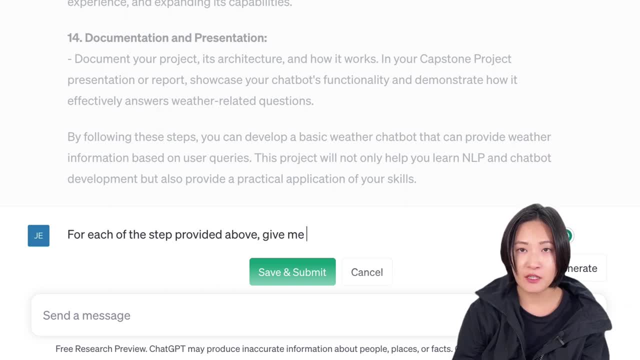 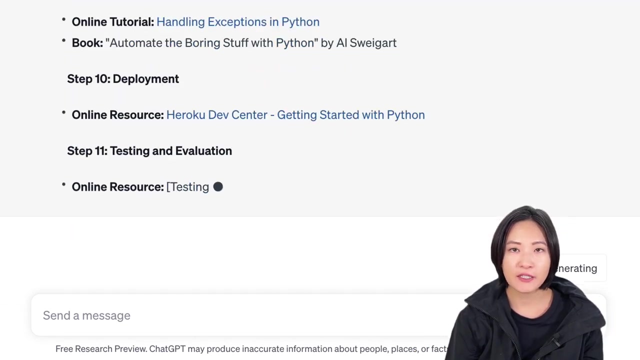 Though, to make it even better, I asked for each of these steps provided above. give me free online resources and books that I can reference to learn the concepts and implement the step. Turn it into an actionable study plan. Then it spit out the resources, which looks pretty good. I do want both of the outlines in one page, So I asked again. 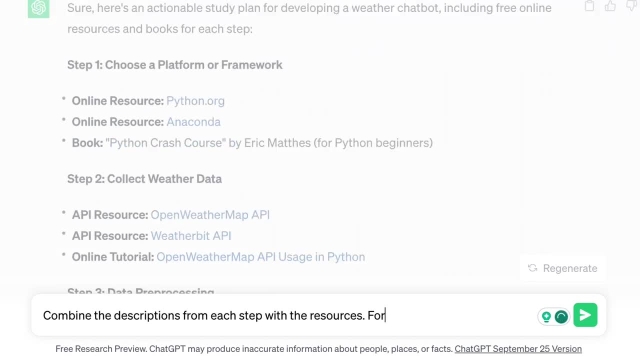 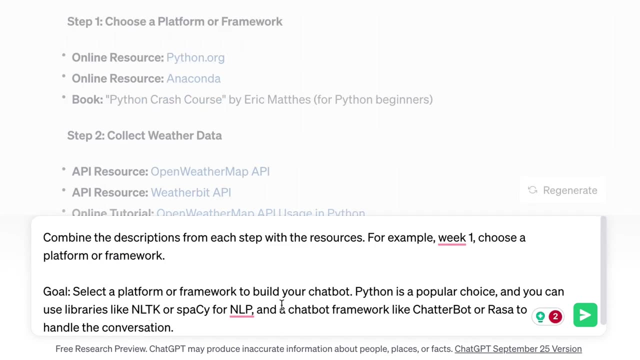 combine the descriptions from each step with the resources. For example, week one: select the platform or framework to build your chatbot. Python is a popular choice and you can use libraries like NLTK or spa, sci or NLP and a chatbot framework like 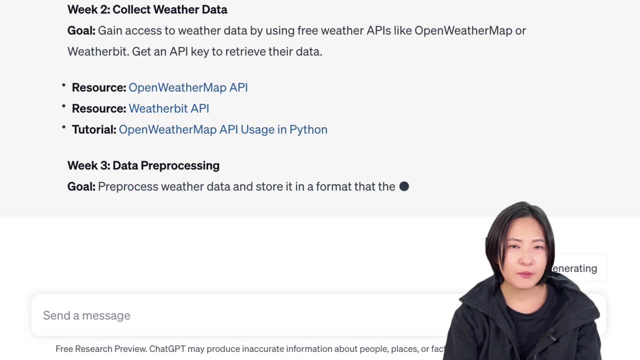 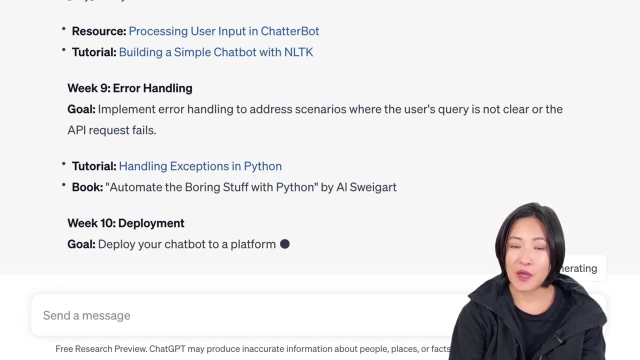 Chatterbot or Rasa to handle the conversation. Sometimes ChatGPT stops in the middle of the answer, but you can prompt it to continue. I'm really loving the new plan. I feel like the concepts make a lot more sense when I'm actually working on hands-on projects. It's kind of like learning math theories without 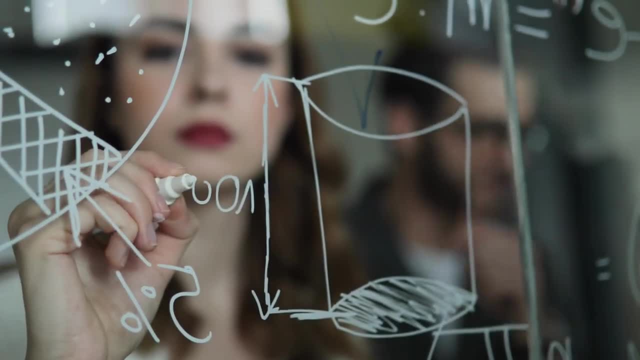 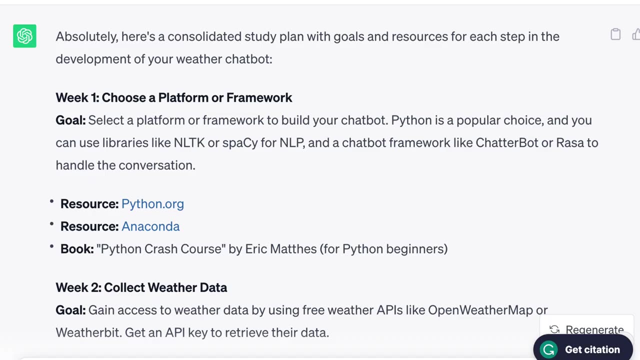 doing the math problems. It's much difficult to soak in the information until you put it into practice. As I read through the plan, I do see that for week one it suggests a Python crash course. Can you become a Python expert in one week? Probably not, but that's totally fine because 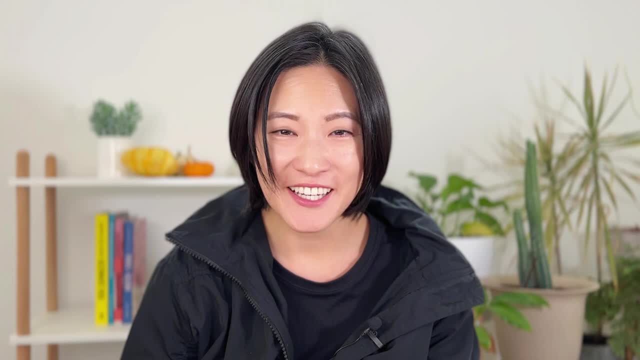 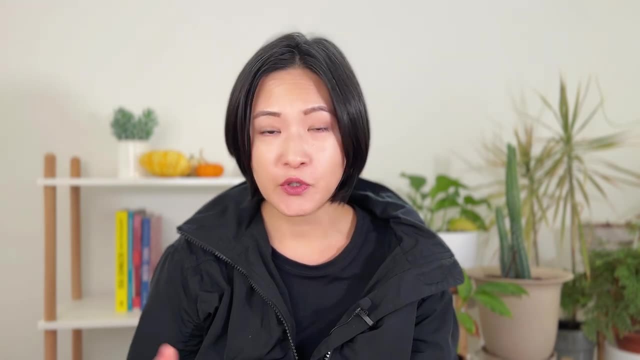 I'm a Python expert. I'm not trying to be a Python expert. I'm trying to create a weather app. The big idea I want to highlight here is that you don't have to be perfect at everything before you begin your project. Many times, as engineers working in the real industry, we're figuring 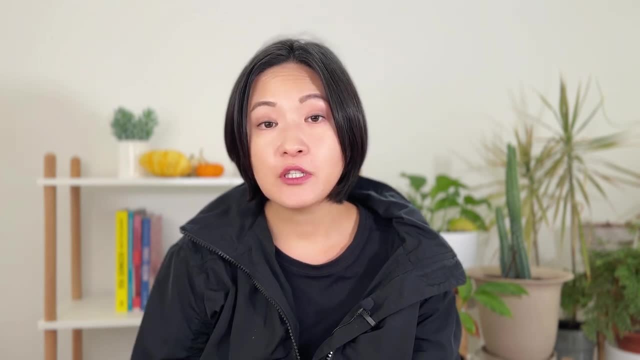 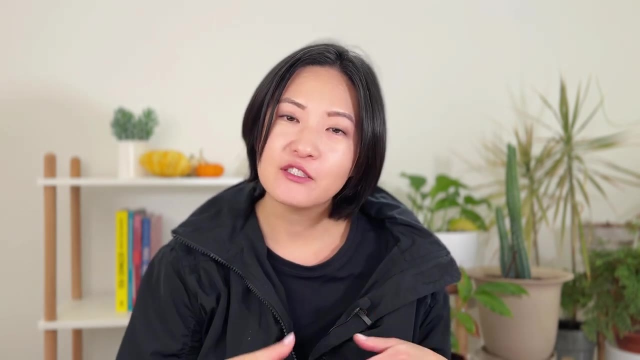 things out as we build them. What really matters is your ability to learn and adapt along the way, So it's more about the journey more than being perfect. So if you're new to Python, for the first week, just focus on setting up your environment so you can get started with. 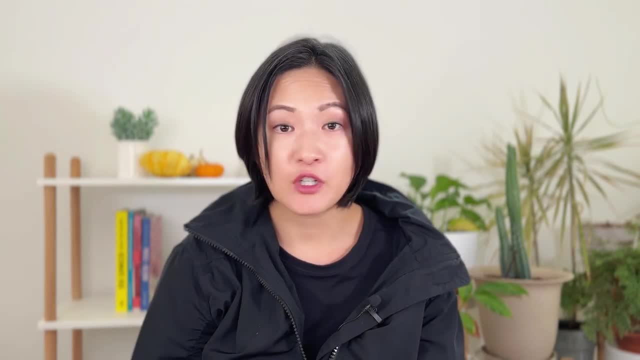 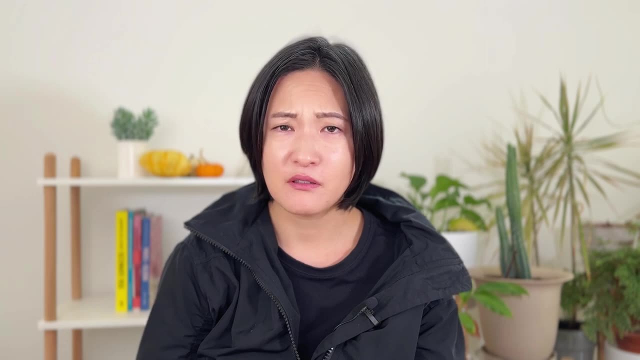 the project. If you have done Python before, spend the week brushing up on new concepts. Step 12, ChatGPT picked Flask for me, but Flask is not a very popular technology right now, So I asked for an edit For step 12,. instead of using Flask, I want to integrate with Facebook Messenger. 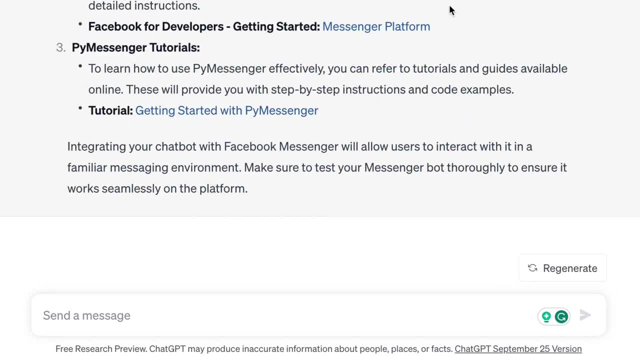 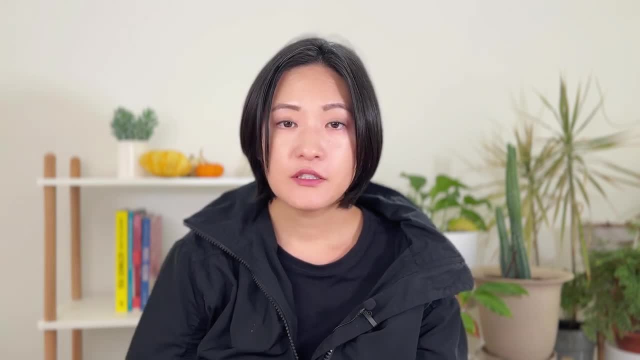 Give me a new recommendation. The new resources for week 12 are much better, So the idea is that you can pretty much do this for each step. Where you feel like you need a little bit more resources, ask again. Similarly for week 14,. it says: document your project, its architecture and how it works. 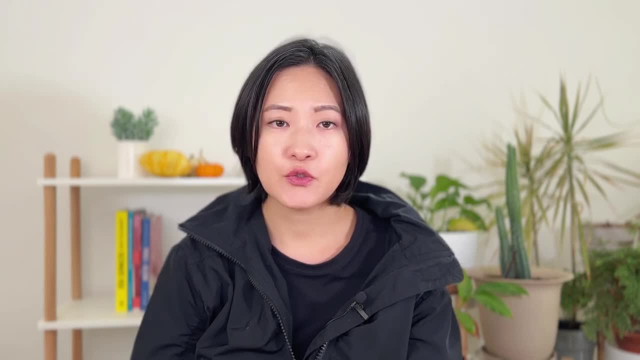 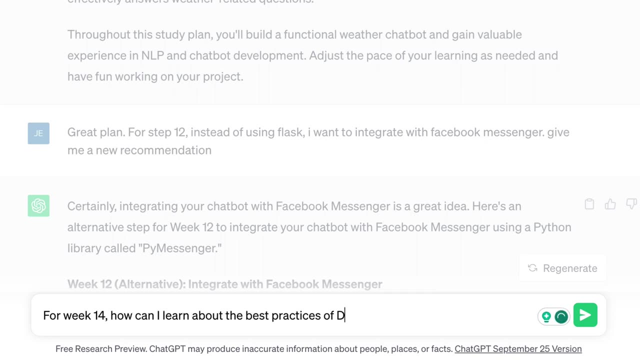 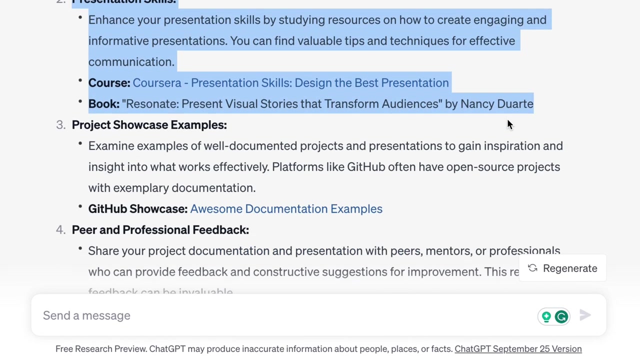 If you plan to work on projects, it makes sense to add them to your Github. So I tried asking. I want to document my project on Github For week 14, how can I learn about the best practices of documenting on Github? It gave me a lot of resources here about Github but it was not.